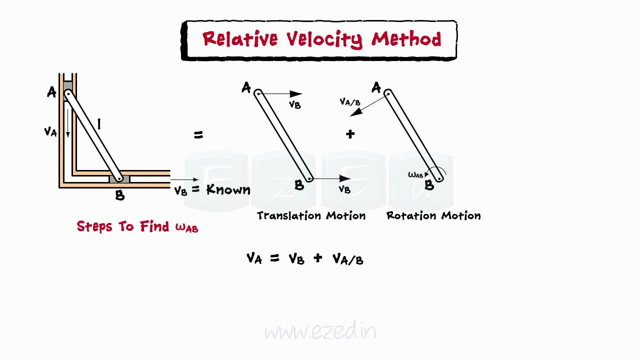 For point A. we will write the relation as shown, Step 5.. Write the relation for the absolute velocity of the translation point. Simultaneously, Draw the vector diagram of the same. From the relation, vab can be found out. 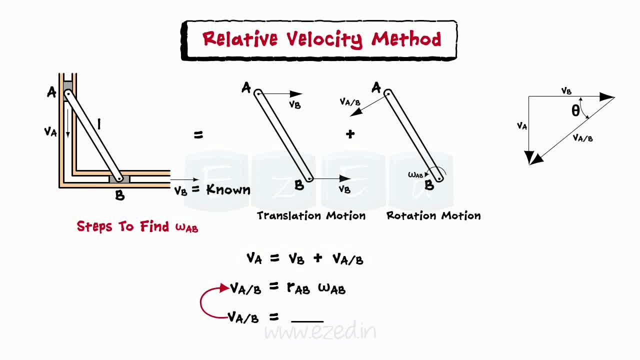 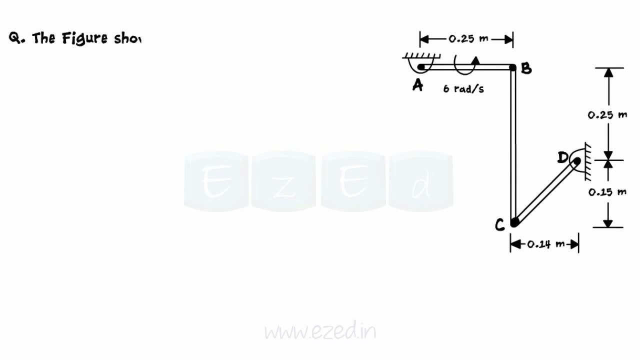 And when we substitute the value of vab in relation for relative linear velocity, we get an angular velocity omega. Let's take an example and solve it by relative velocity method. The figure shows three bars: ab, bc and cd. Internally, pin connected at b and c and externally hinge. 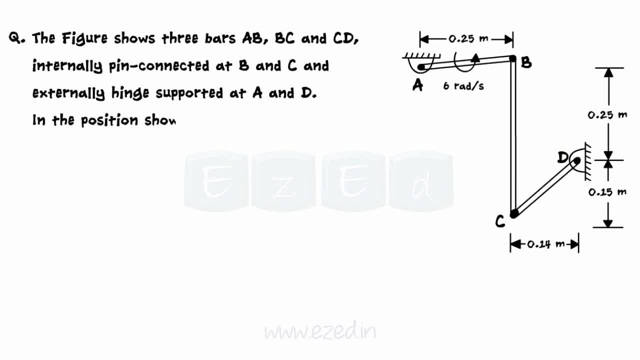 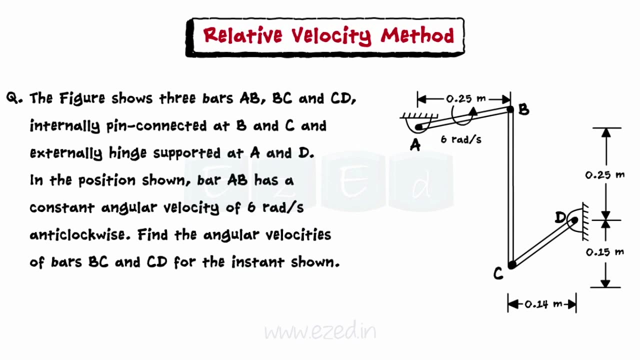 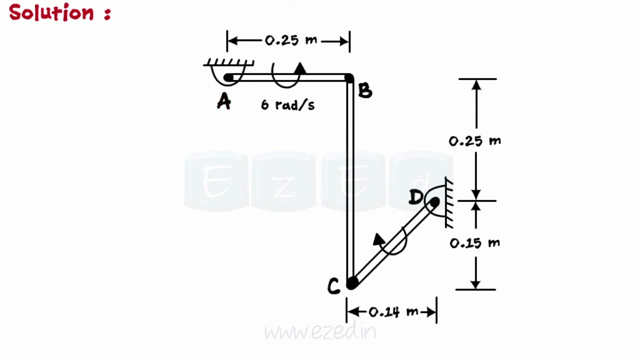 supported at a and d. In the position shown, bar ab has a constant angular velocity of 6 radians per second, anti-clockwise. Find the angular velocities of bars bc and cd for the instance shown Here. rod ab performs rotation motion about a. 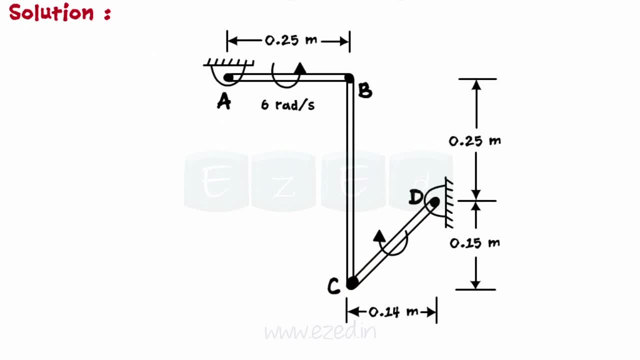 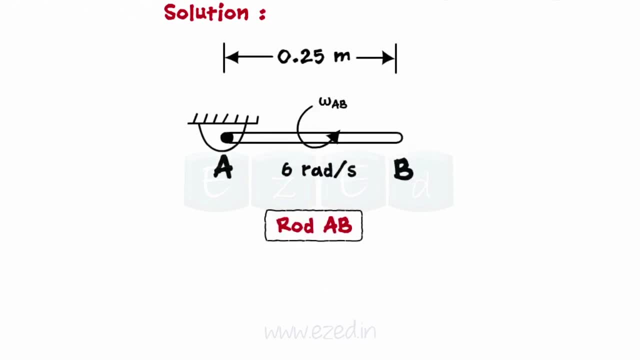 Rod cd performs rotation motion about d And rod bc performs general plane motion. Consider rod ab. Rod ab rotates about a point a, So direction of velocity at point b would be perpendicular to the radial distance ab. Therefore, using relation between linear velocity and 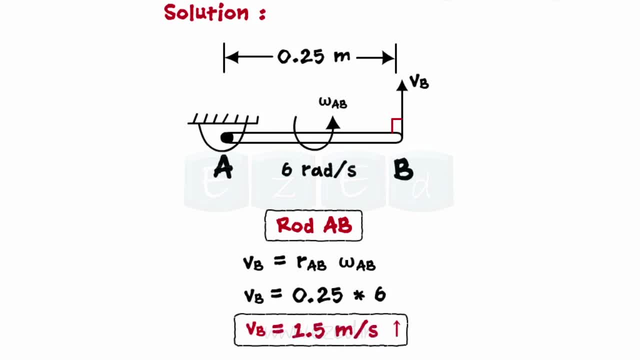 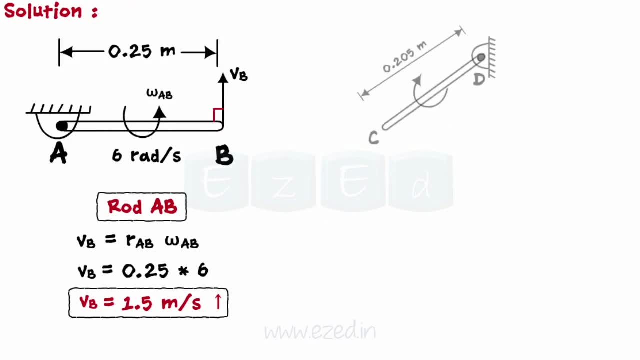 angular velocity. on substituting the values, we get velocity of vb. The velocity of vb is equal to the angular velocity at point c. Consider rod cd. Rod cd rotates about a point d, So the direction of velocity at point c would be perpendicular. 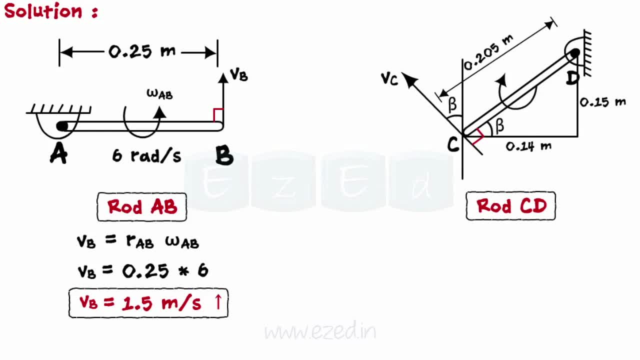 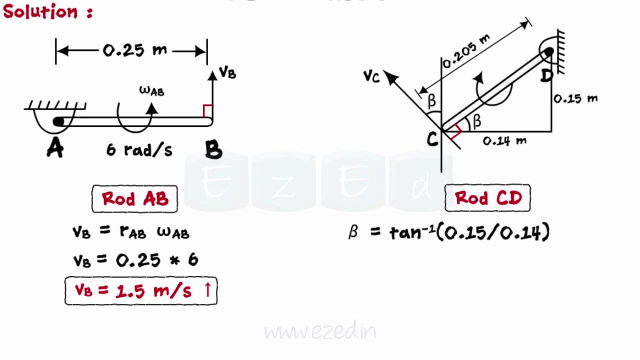 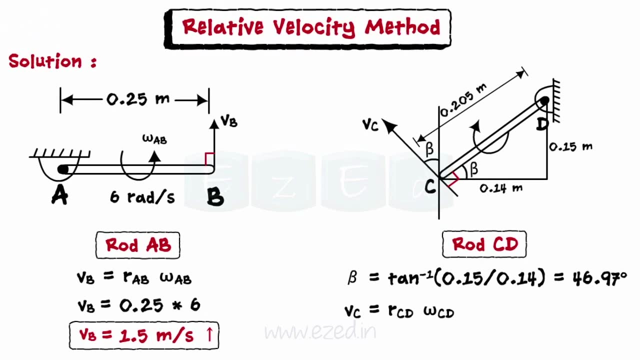 to the radial distance, cd. Let beta be the angle made by vc with the vertical. From the geometry, the value of beta is 46.97 degree. Therefore, using the equation between linear velocity and angular velocity on substituting the values, we get equation 1.. 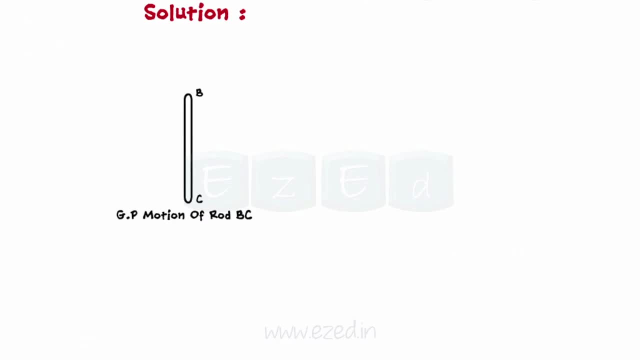 Consider general motion of rod bc. For general plane motion we will use relative velocity method. Step 1. Locate the point whose magnitude and direction is known. Here velocity of point b is known. Step 2. Locate a point whose direction is known, that is, point c. 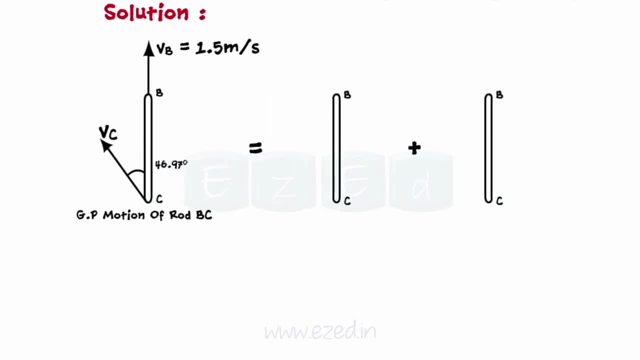 Step 3.. Now divide the motion of the body as sum of translation and rotation motion. Translate the body with the translating velocity, that is, vb, and rotate it about a fixed point b, Step 4.. Write the relation for the absolute velocity of the translation point. 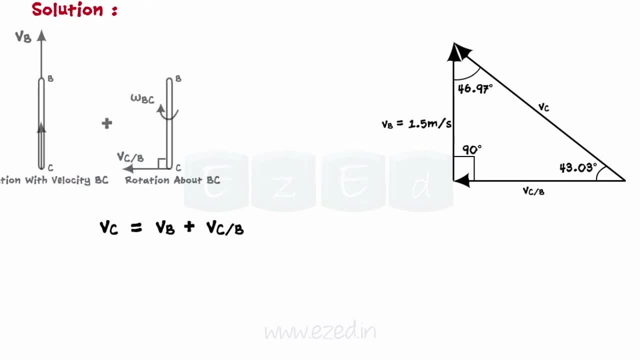 Simultaneously draw the vector diagram of the same. On solving the triangle, we get vb. On the triangle, we get velocity at point c as 2.2 meters per second and relative velocity of c with respect to b as 1.61 meters per second. 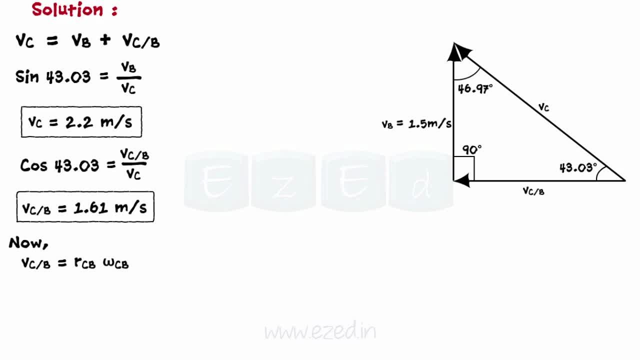 Step 5.. Write the relation for the relative linear velocity of translating point. On substituting the value, we get an angular velocity of rod cb, Step 6. Now, substituting the value of vc, we get a warsaw of the current velocity. 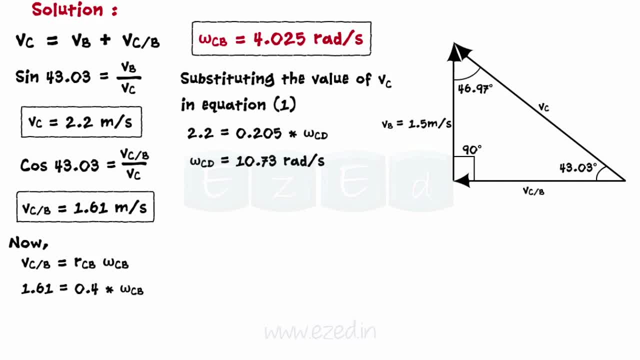 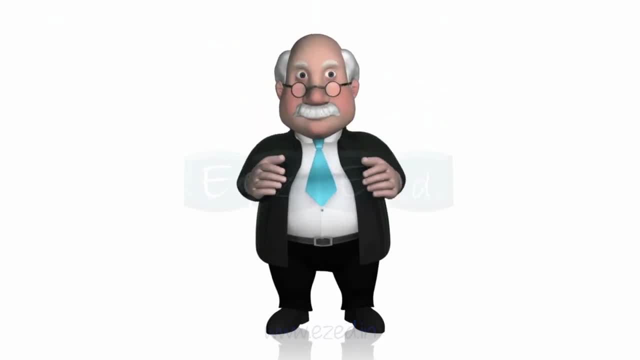 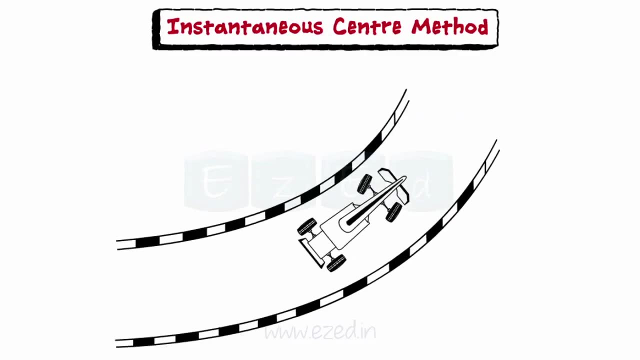 Step 7.. In equation 1, we get angular velocity of rod CD. Seriously, pay attention, This is important. Instantaneous center is defined as the point about which the general plane body rotates at the given instant. The instantaneous center of rotation lies at the intersection of the perpendicular to the velocity. 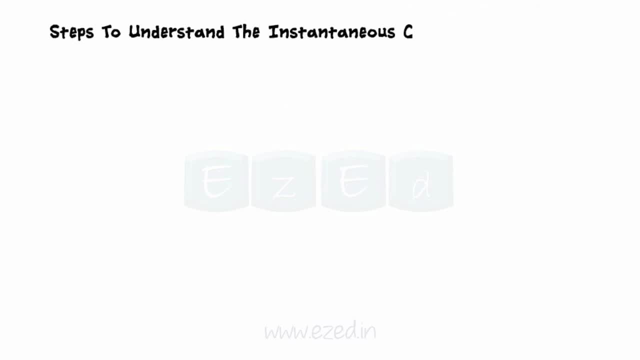 Let us see steps to determine the instantaneous center. Consider the mechanism of a rod attached to a slider. We have the given velocity of VA and we have to find an angular velocity of rod AB at the given instant. Step 1. Locate a point whose magnitude and direction of velocity is known and another point whose direction of velocity is known. 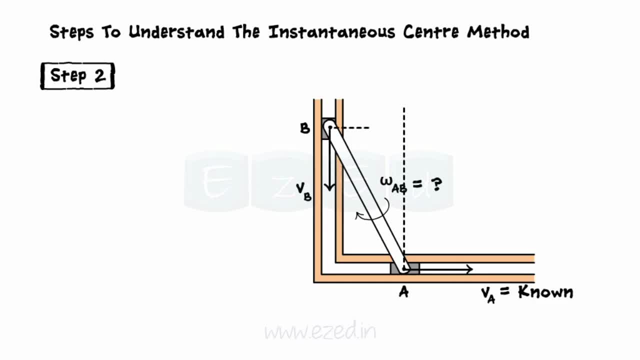 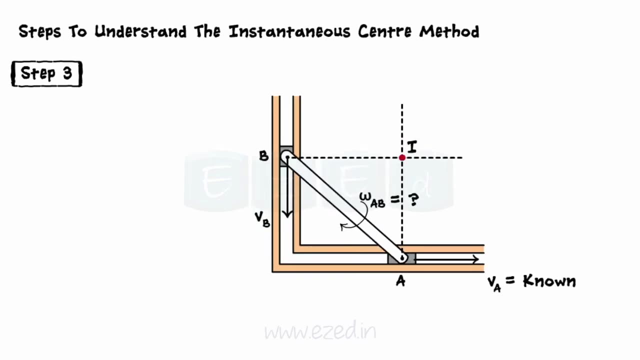 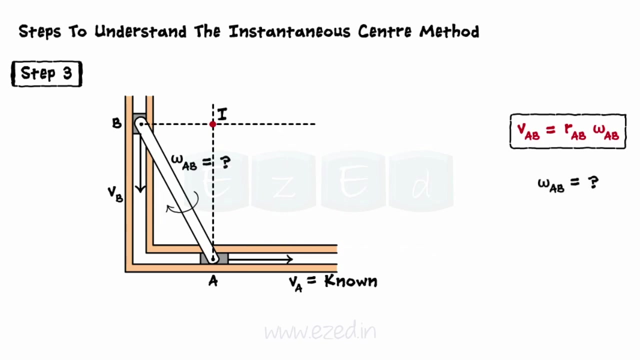 Step 2. Draw the perpendicular to the direction of velocities and extend them to intersect at a point. Call the point as I. Step 3. Point I is the center of rotation of the general plane body at the given instant. On using the relation V equals R omega, the angular velocity of rod AB can be found out: 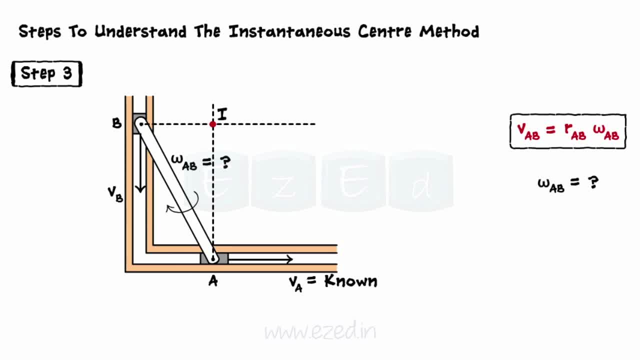 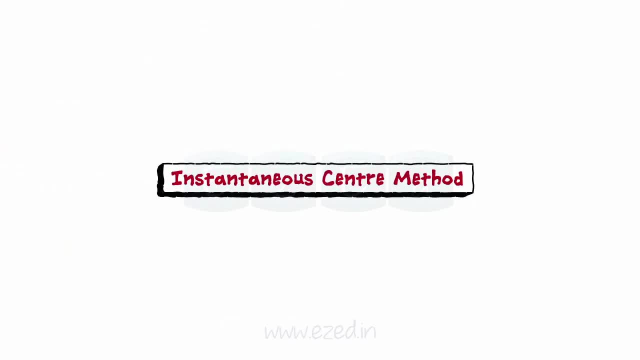 Once the angular velocity is known, the angular velocity of rod AB can be determined by the position of another velocity. Let us solve a problem on instantaneous center method. The figure shows collar B, which moves up with a constant velocity of 3 meters per second. 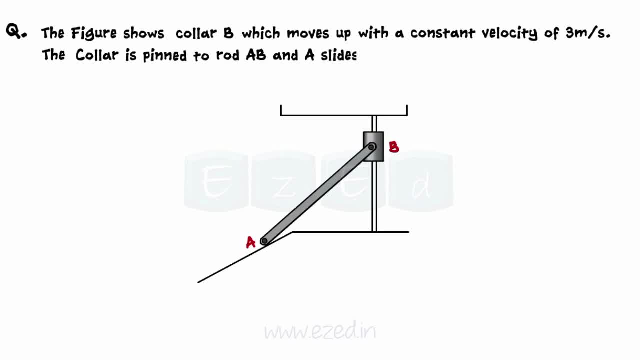 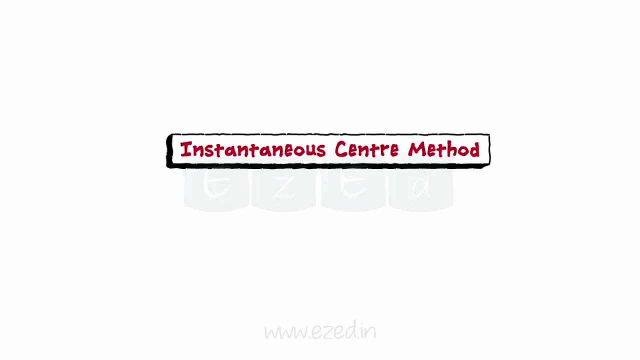 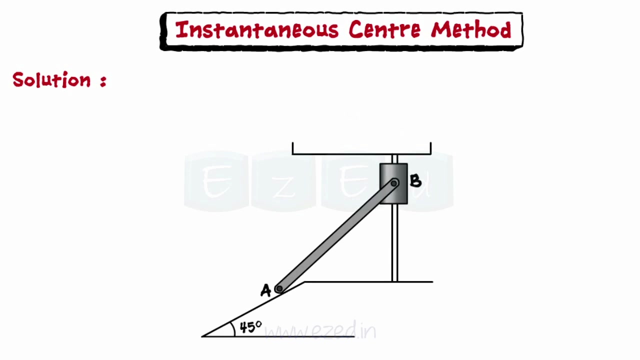 The collar is pinned to rod AB and A slide freely against a 45 degree sloping ground, For this instant determine the angular velocity of the rod and velocity of end A of the rod. The system consists of two bodies in motion. Rod AB performs a general plane motion and collar B performs a rectilinear translation motion. 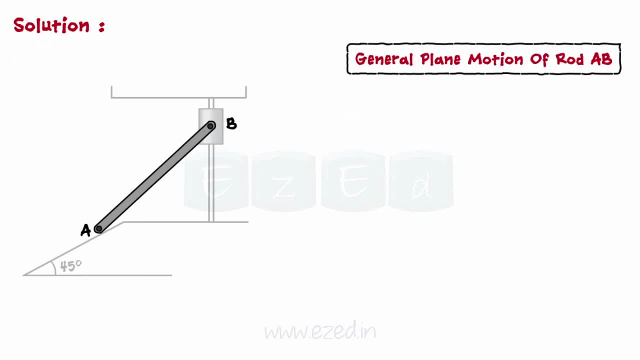 Considering a general plane motion of rod AB using instantaneous center method, Step 1.. We know velocity at point B, that is 3 meter per second. Also, the direction of velocity of point B and direction of velocity at point B are the same. 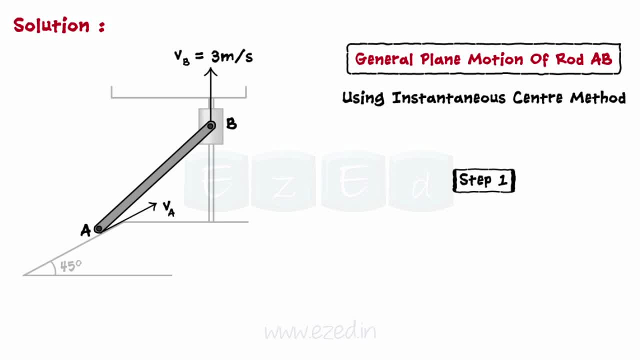 The direction of velocity of point B and direction of velocity at point B are the same. Also, the direction of velocity of point B and direction of velocity at point A are the same. Step 2. Draw the perpendicular to the direction of velocity at point A and B. 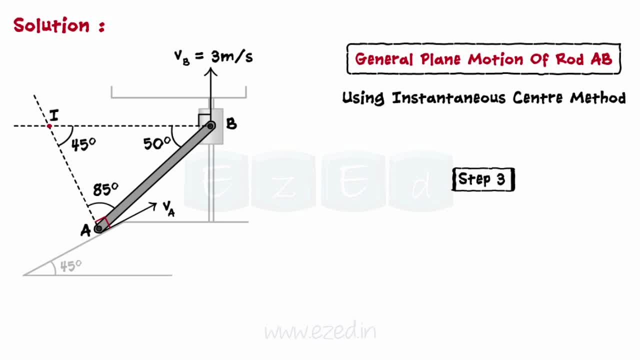 Let the point of intersection be I, Step 3. From the geometry, the radial length can be found out using the sine rule to solve triangle ABI. On evaluating, we get the radial distance. Step 4. Use the relation between the linear velocity and an angular velocity at point B. 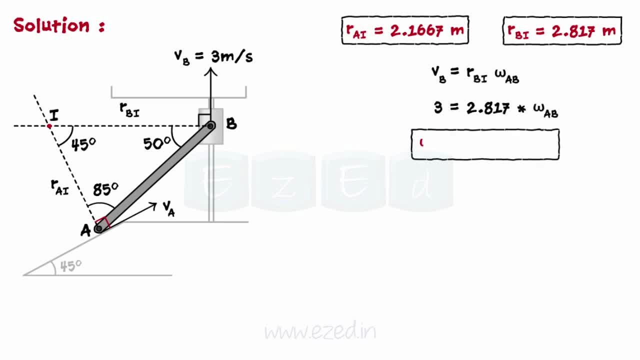 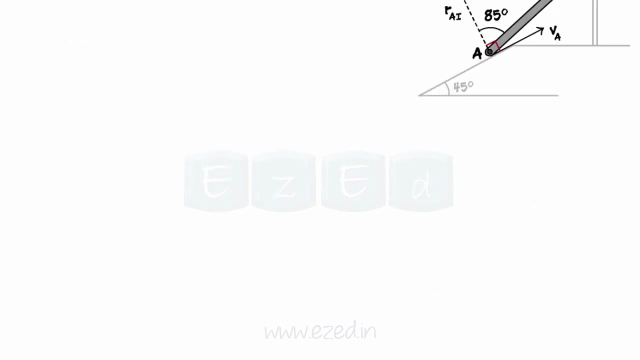 On substituting the values, we get angular velocity of rod AB as 1.06 radians per second. Now use the relation between linear velocity and an angular velocity at point A. On substituting the values, we get the velocity at point A as 2.3 meters per second.